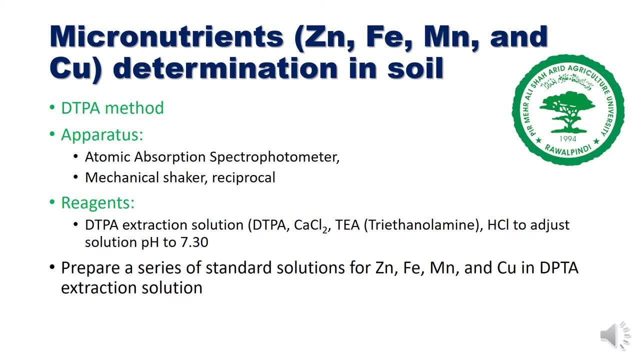 agents, which combines with free metal ions in the solution to form a soluble complexes of metals. This is a very important and useful method for determining the micronutrient, particularly in the alkaline soil. The apparatus we need for this experiment is atomic absorption spectrophotometer, mechanical 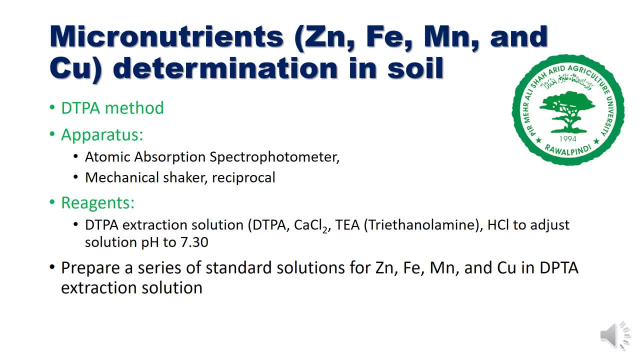 shaker and the glassware. The reagents we need for this experiment are most important. one is the DTPA extraction solution. How we can prepare this DTPA extraction solution I will show you in the video demonstration. But to prepare DTPA extraction solution we need DTPA and calcium chloride. 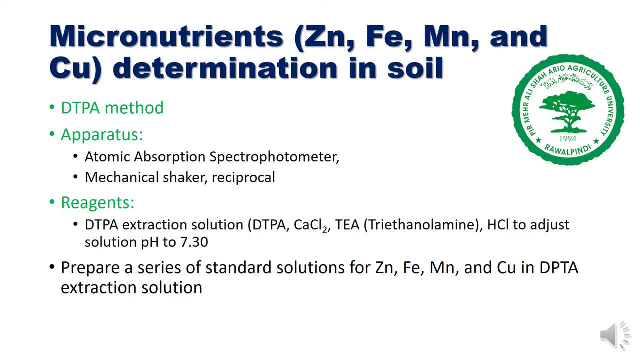 We need to mix them in a beaker. We need 1.97 g DTPA and 1.1 g calcium chloride to dissolve in distilled water and then transfer it to one liter volumetric flask. We also need to prepare DEA, triethanol amide. 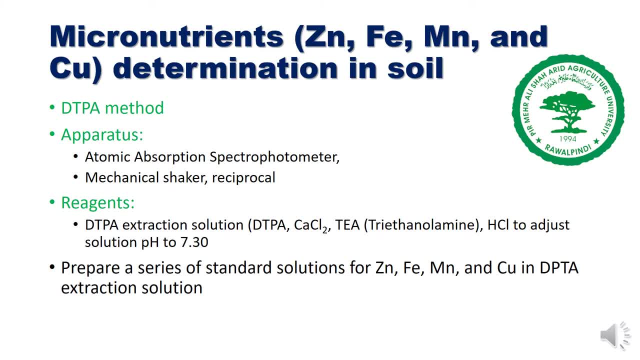 This DTPA analysis WHAT we want to prepare: DEA, dry ethanol Amine. Dea is made from a day of medicine weighing 14.92 gram or 13.3 in the liquid form, transferred with the distilled water into a one liter flask and then bring it volume to up to the mark and we will mix all these reagents and 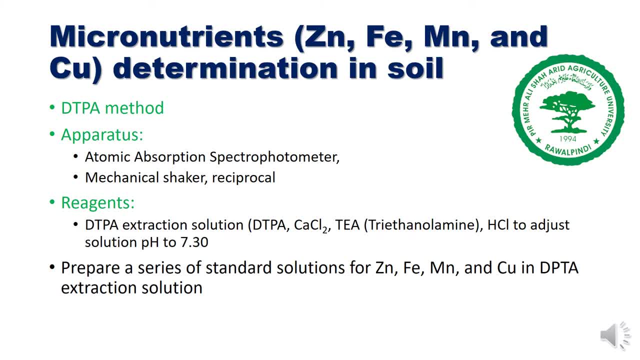 we need to adjust their pH exactly to two point eight, seven point three with HCl, six normal HCl- and this btp extraction solution will contain 0.005 molar DTPA, 0.1 molar tea and 0.1 molar. 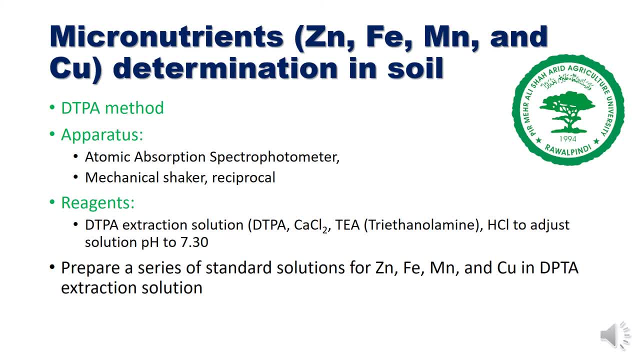 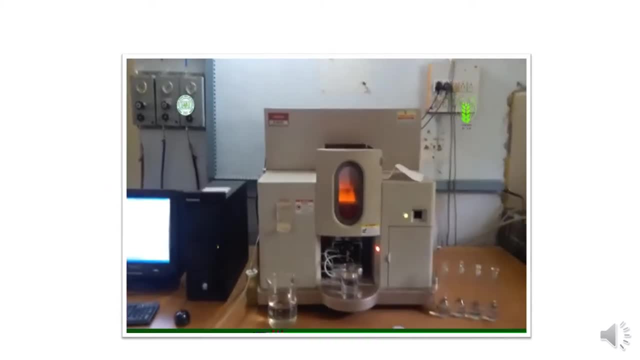 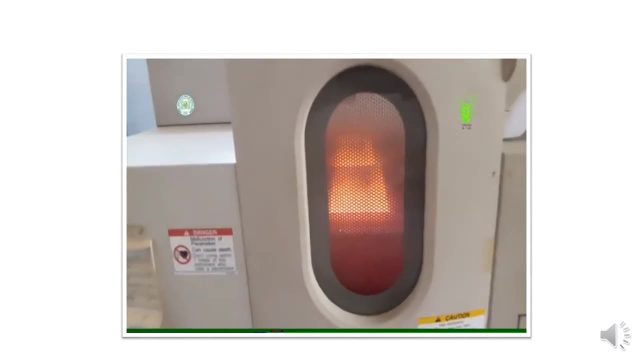 calcium chloride. we also need to prepare a serial, a series of standard solution for each micronutrient by using their respective salt. here I'm going to demonstrate you about how we we need to determine the micronutrient from a particular soil. for this, I already mentioned, we need atomic 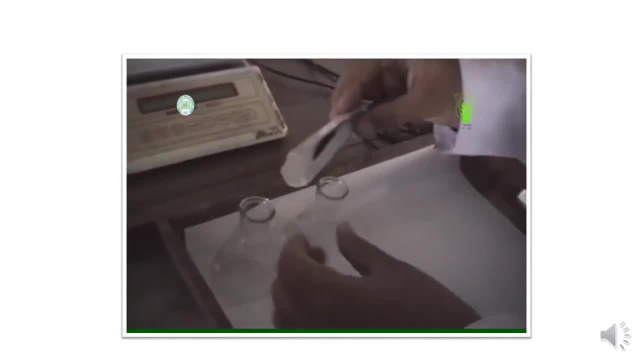 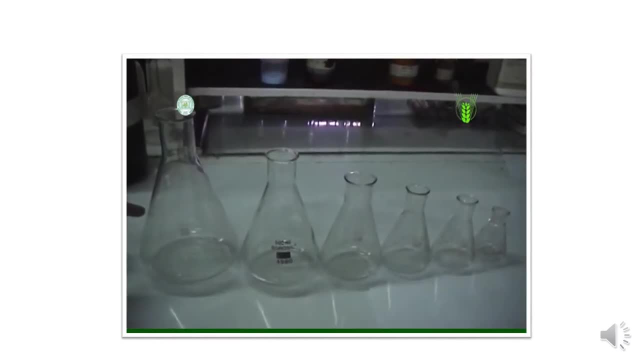 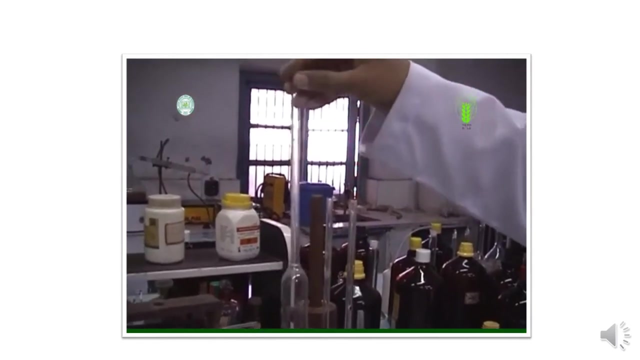 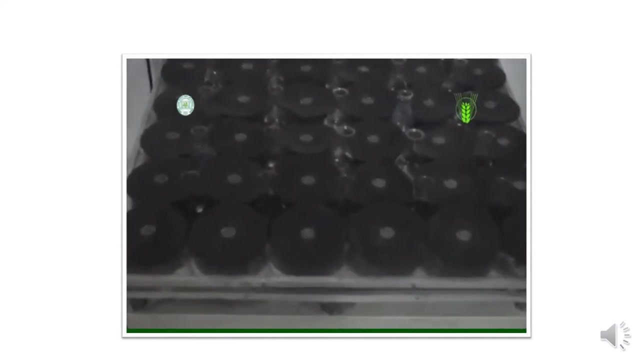 absorption in the picture you are witnessing here is related is of the atomic absorption spectrophotometer. this is very important instrument and through which we can measure all the micronutrients that I mentioned, like iron, zinc, manganese and the copper. we also need the atomic absorption spectrophotometer with which we can measure all the micronutrients that I mentioned, like iron, zinc, manganese and the copper. we also need 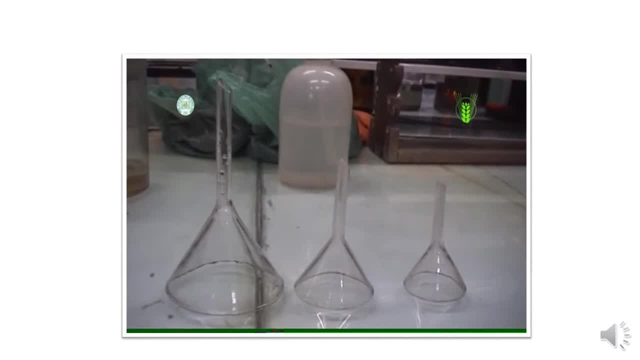 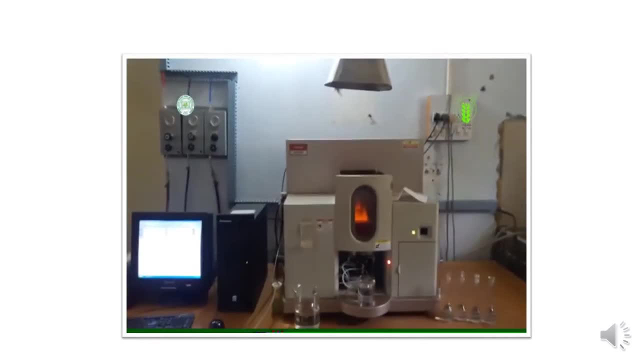 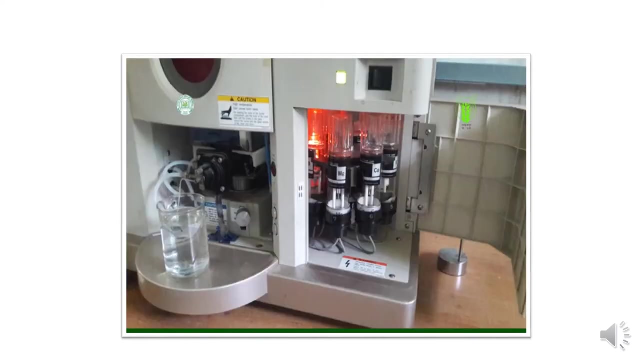 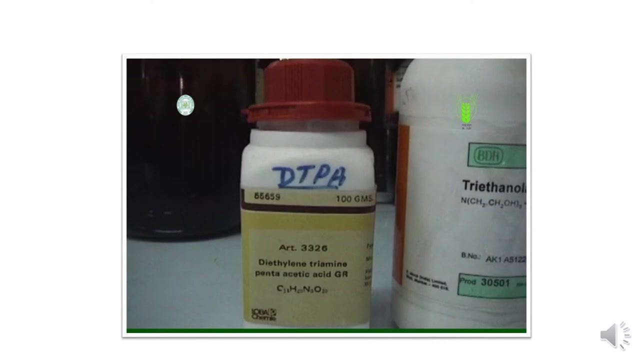 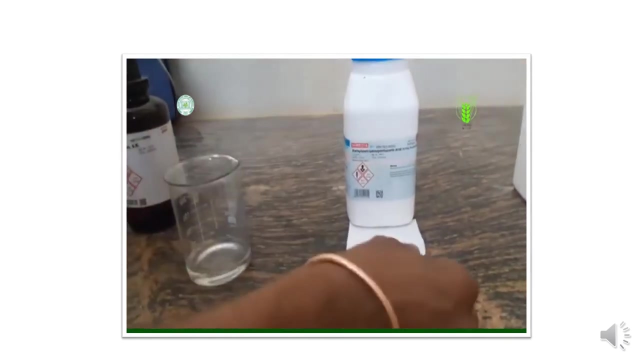 electronic balance as well as we need flasks different, the flask with different capacity and the volumes we need for the shaking purpose. we also need the pipette and also we also be using the mechanical shaker as a broker. we also need the filter paper and the funnels, the bottles, different for 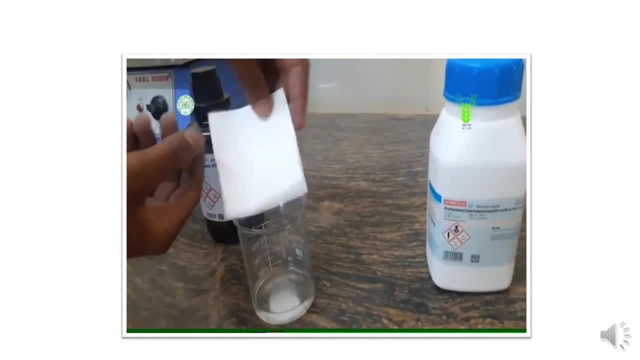 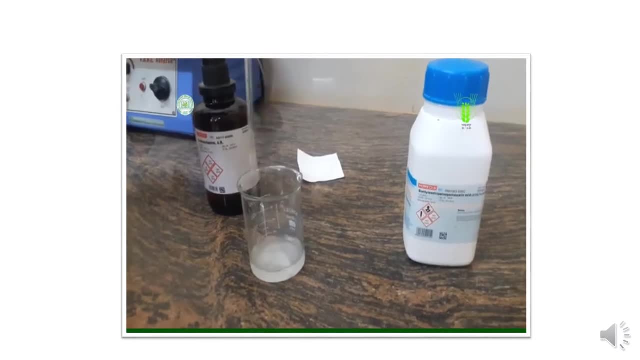 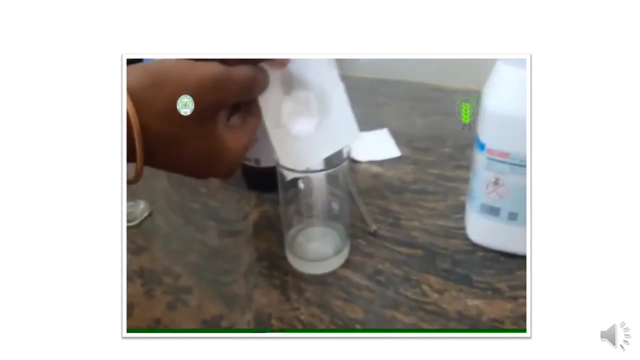 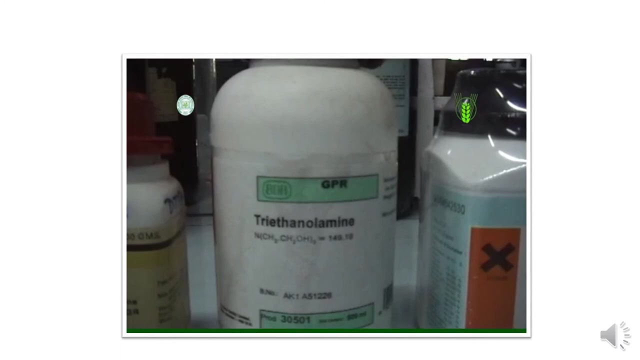 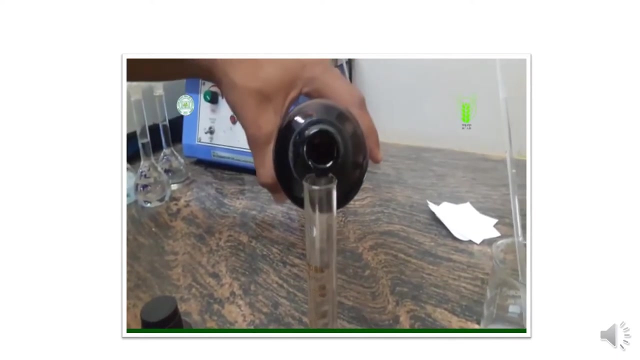 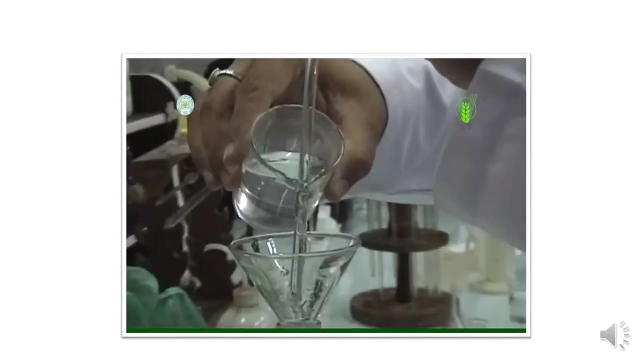 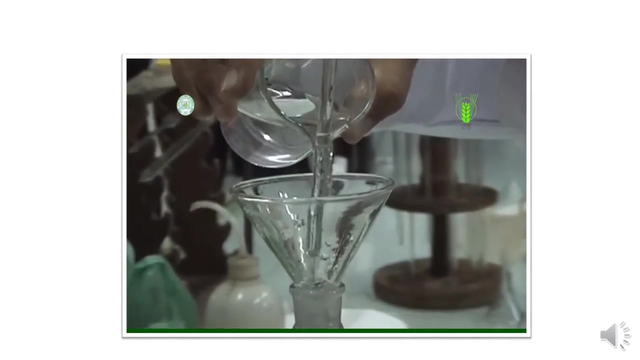 distilled water. here, before starting the experiment, we must run the atomic absorption so it's be ready for the for the analysis of different micronutrients. we also, as I already mentioned, we need different reagent to prepare the DTPA extraction solution, try ethanol amine. 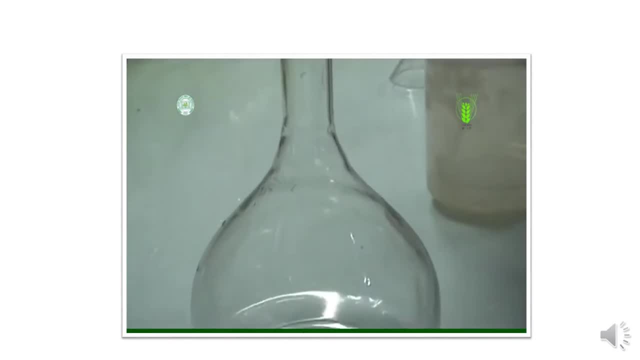 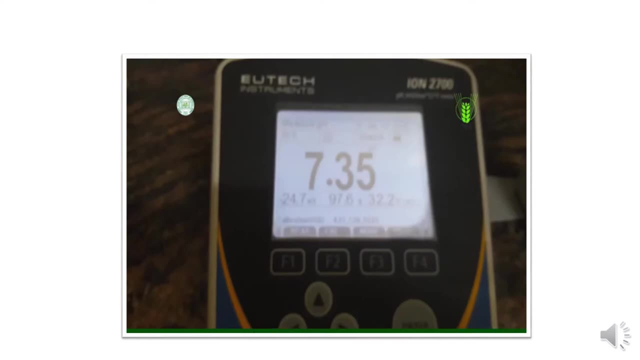 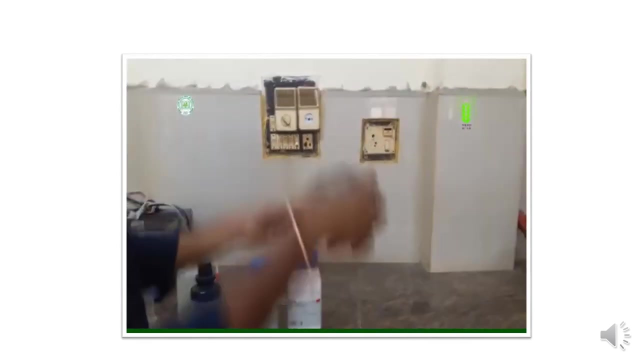 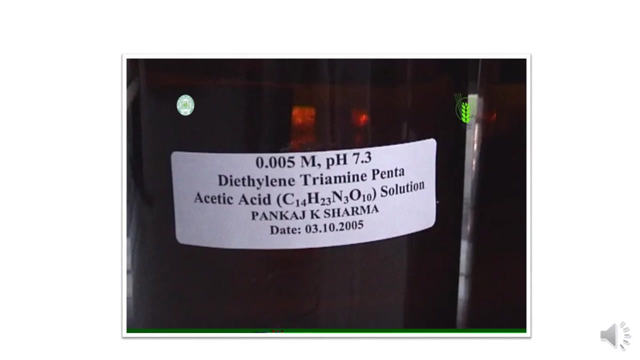 TEA that I already mentioned. we also need to prepare this by adding 13.3 ml and making its volume to up to mark, to a one letter, and its concentration will become 0.1 molar TEA. that's how we are going to prepare it. we also need the pH meter because in while 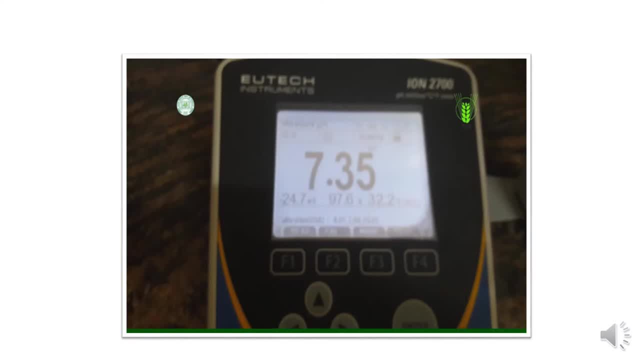 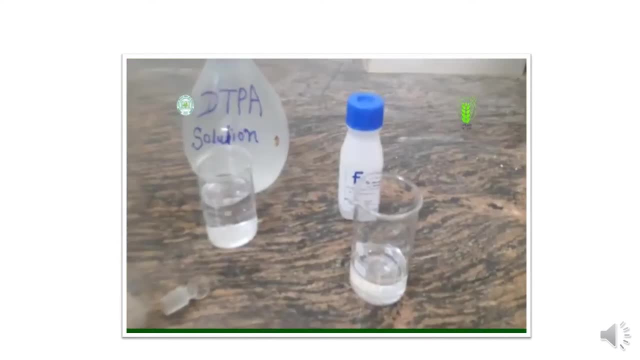 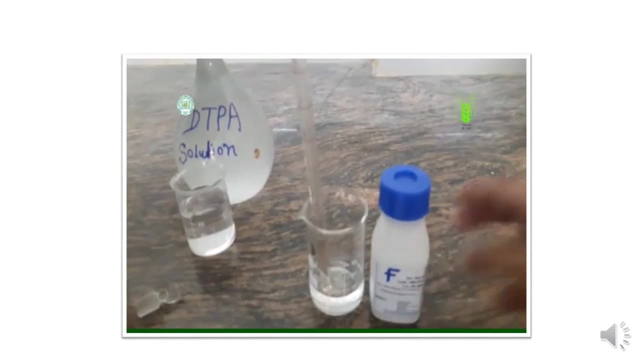 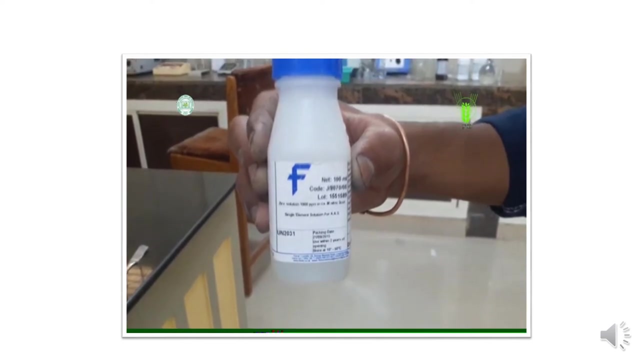 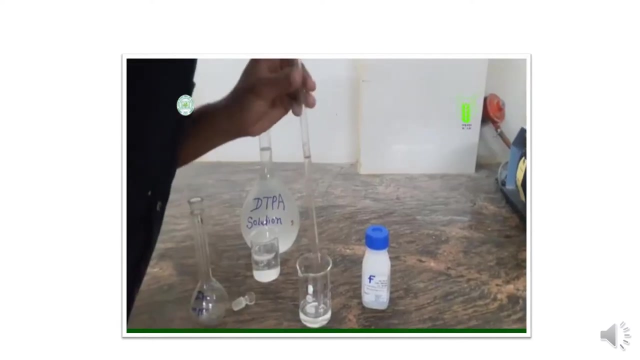 preparing the ttp extraction solution, we need to adjust its pH after mixing DTPA and calcium chloride and try a mine, try ethanol mine, and we must use this щw. the stopped action of these solute välong may mut, And we must adjust its pH exactly 7.35.. 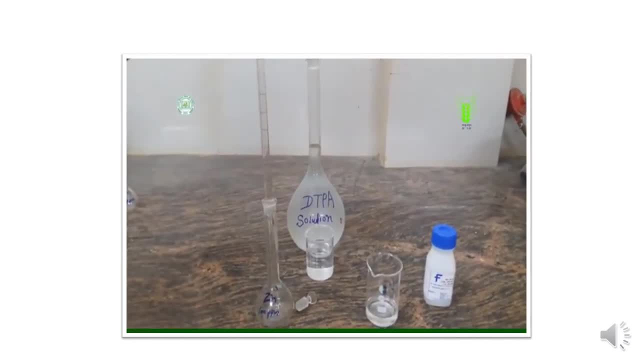 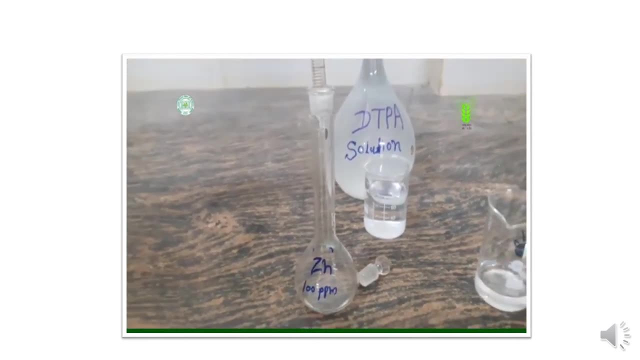 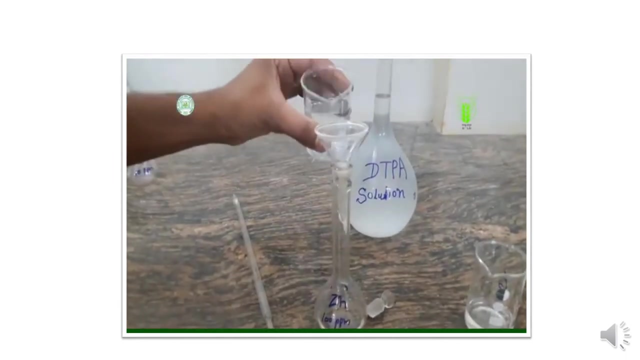 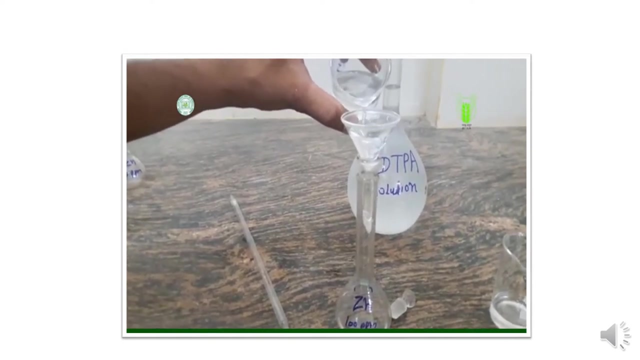 After adjusting the pH of DTP extraction solution. we need to prepare stock solutions of different micronutrients. We need to prepare a separate stock solution for each micronutrient like iron, zinc, copper, manganese. We need to prepare a series of standard solutions for each micronutrient. 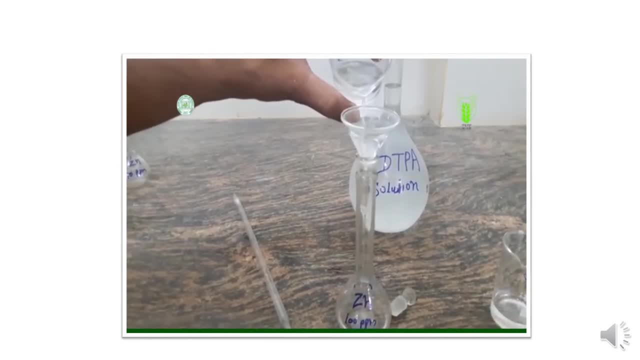 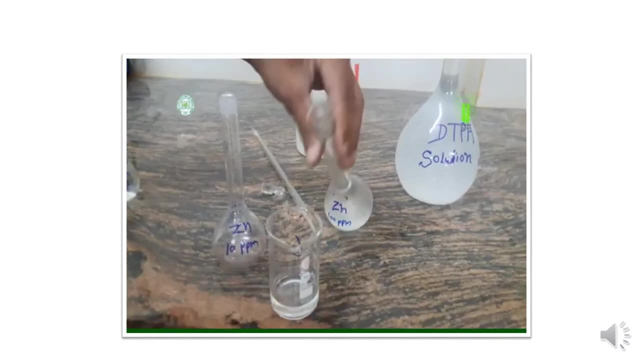 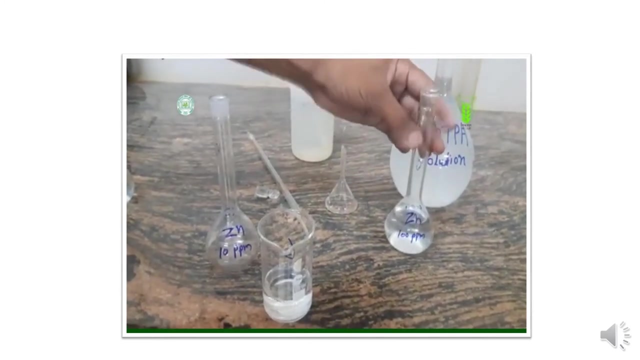 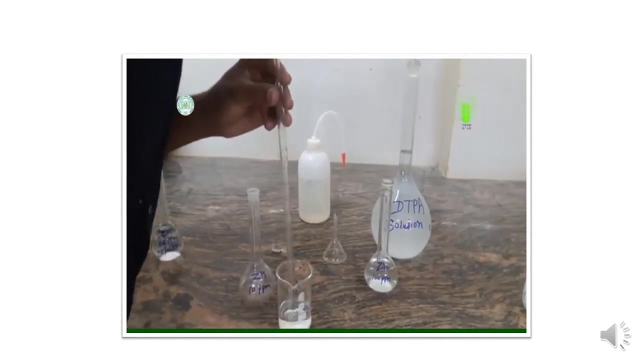 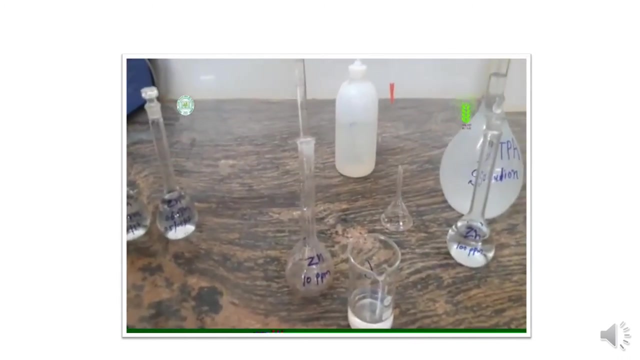 To prepare a series of standard solutions for zinc, we need to prepare a stock solution of 100 ppm. First we need to dilute the 100 ppm stock solution and pipe a 10 ml diluted solution into 100 ml flask and then dilute to a volume DTP solution. 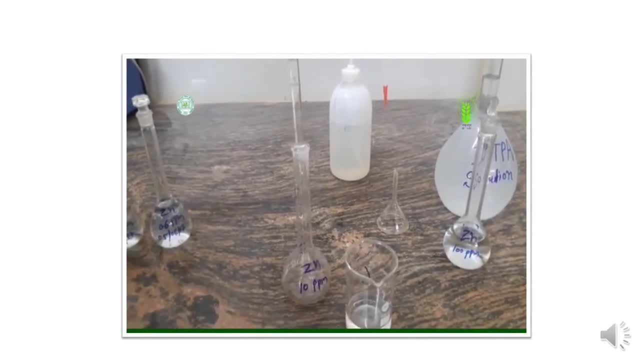 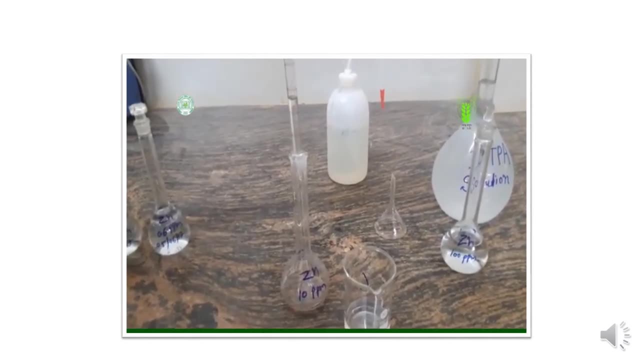 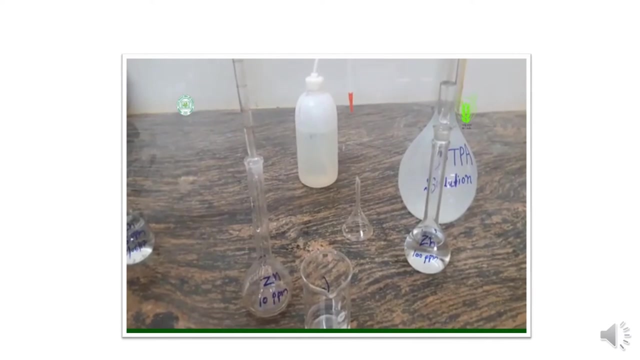 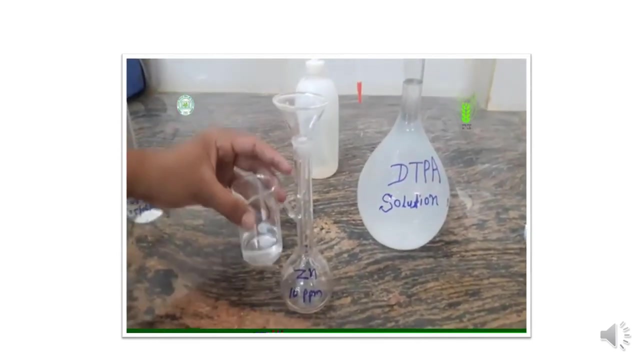 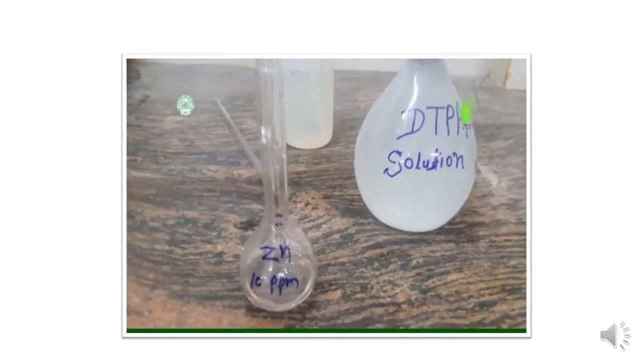 This solution will contain 10 ppm zinc. Then pipe it. We need to dilute the 10 ml flask into 50 ml flask and then dilute to a volume DTP solution. This solution will contain 0.1,, 0.4,, 0.8,, 1.2,, 1.6 and 2 ppm zinc respectively. 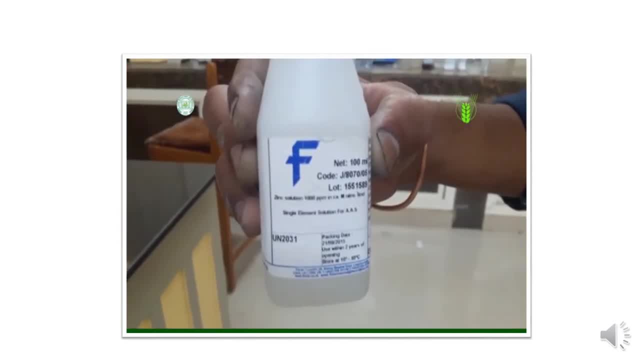 So in this video you can see a different series of stock solutions. We need to prepare a series of standard solutions for each micronutrient like iron, zinc, copper, manganese. To prepare a series of standard solutions for zinc, we need to prepare a syringe of. 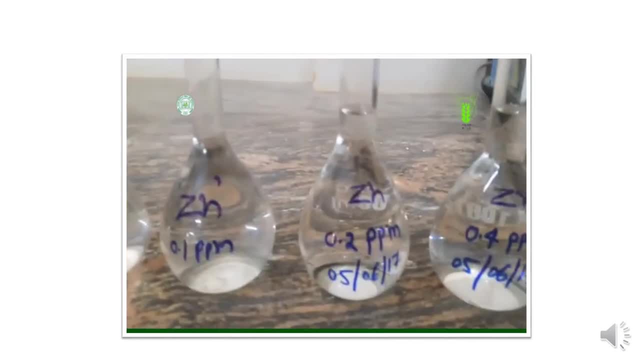 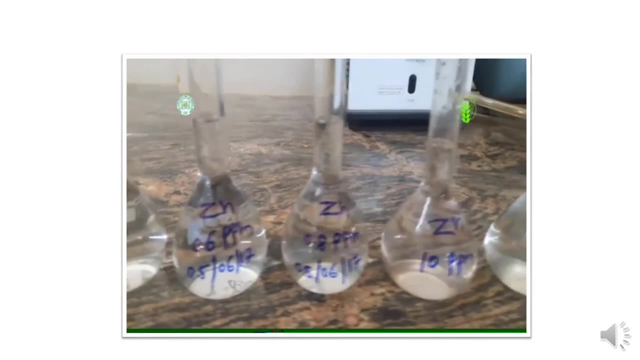 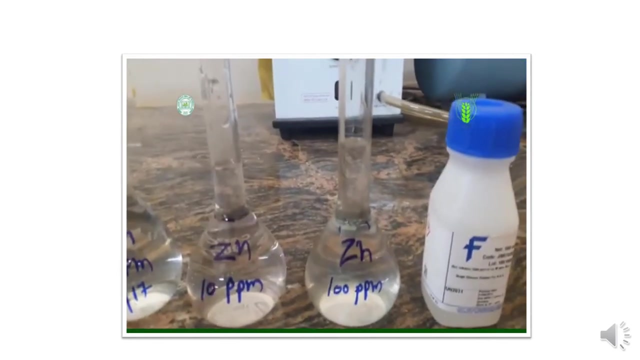 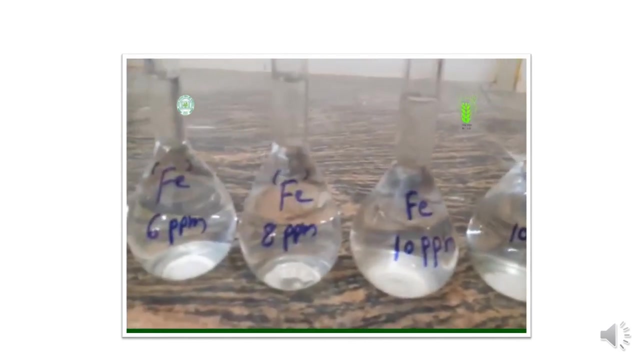 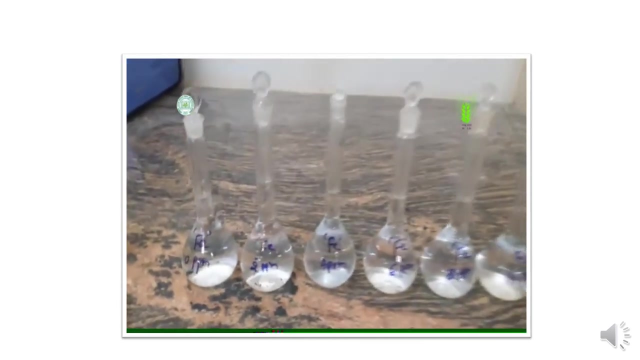 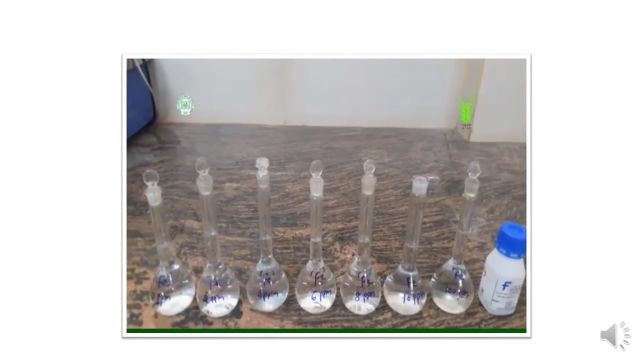 bicarbonate of ethanol to dilute the bes Alfredo CO keep 500 mL of gleichen cies for vitamin C. heel easy avier to prepare the commercial or commercial 박 a- ppm. we can find the commercially available stock solution. thousand ppm of star solution can be. 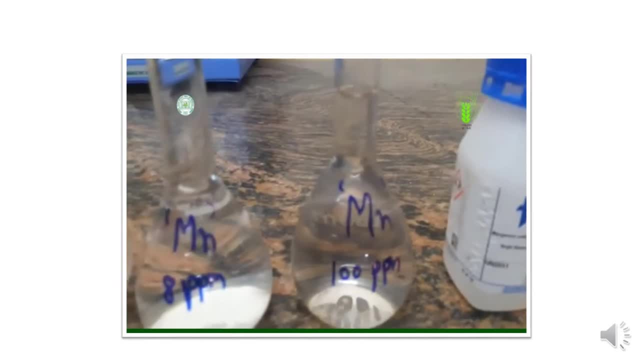 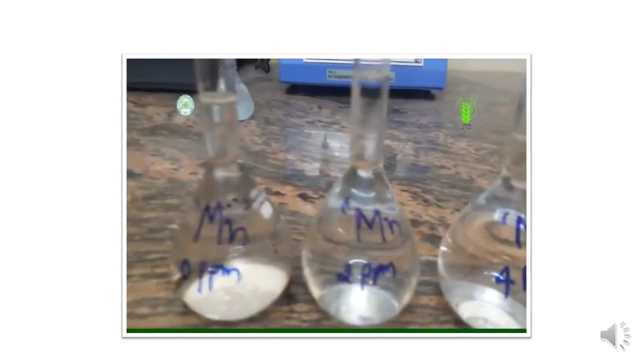 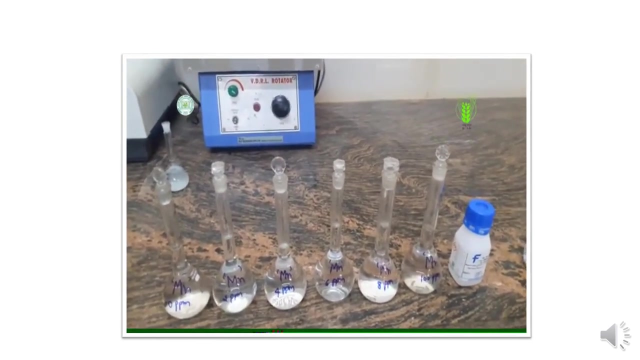 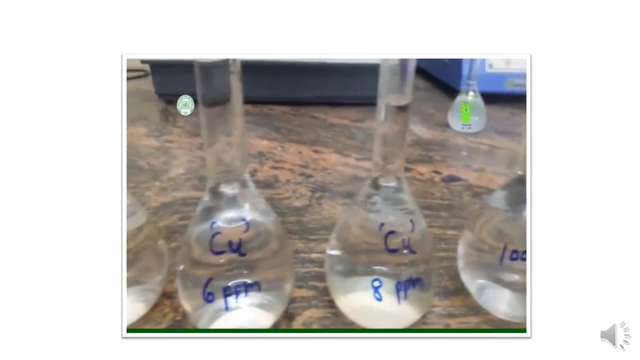 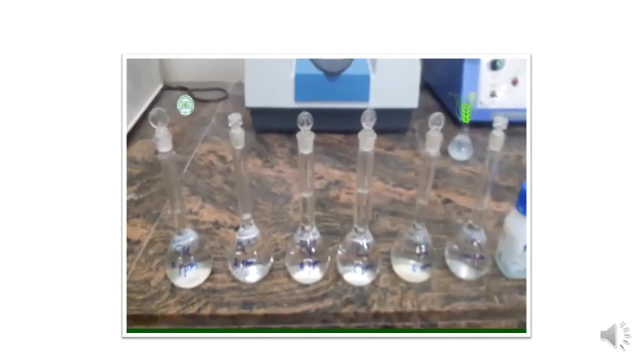 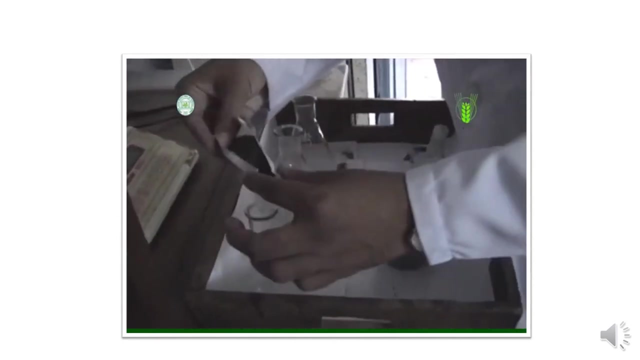 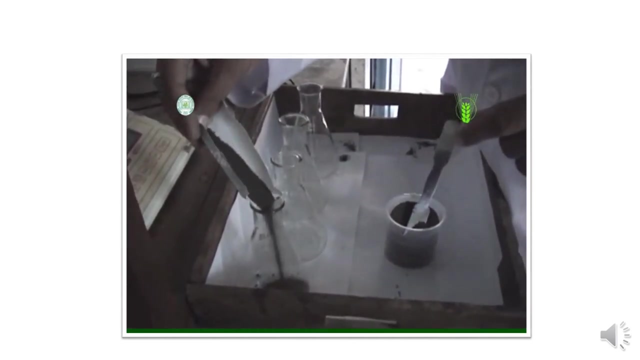 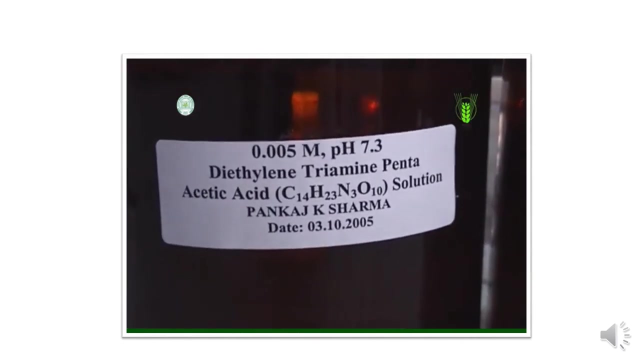 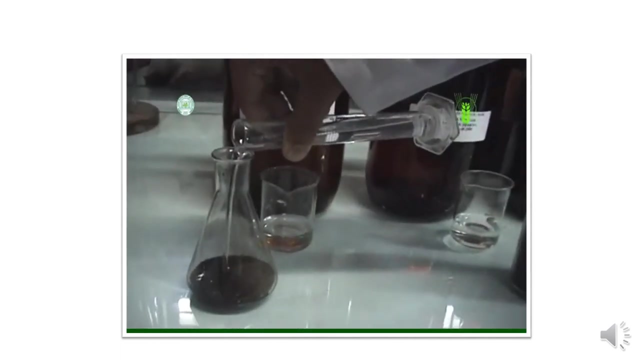 can be purchased from the market and you can prepare by yourself. similarly, like zinc, we can prepare the iron solutions. a different series of standard solutions will be prepared and, as already shown in this video, similarly the manganese standard solution will be prepared, and copper as well. so the first step is we need to take. 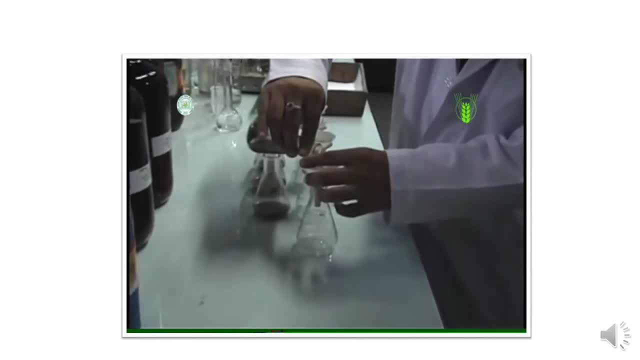 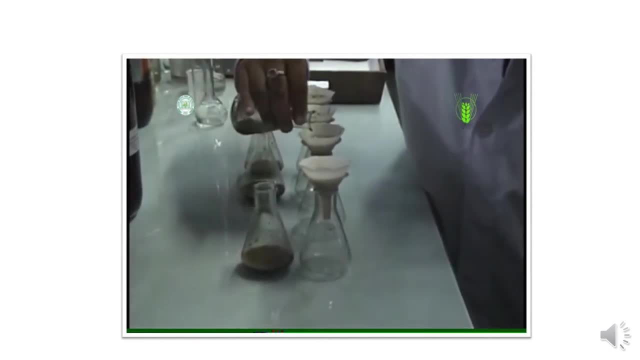 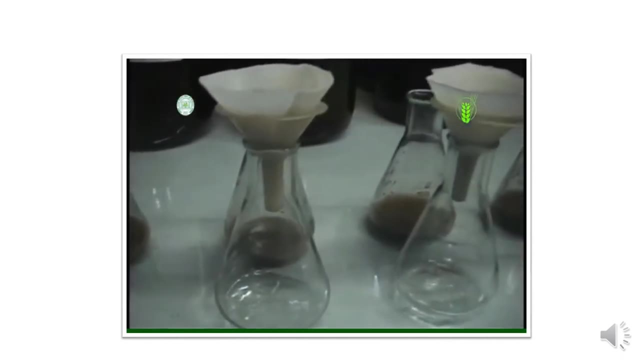 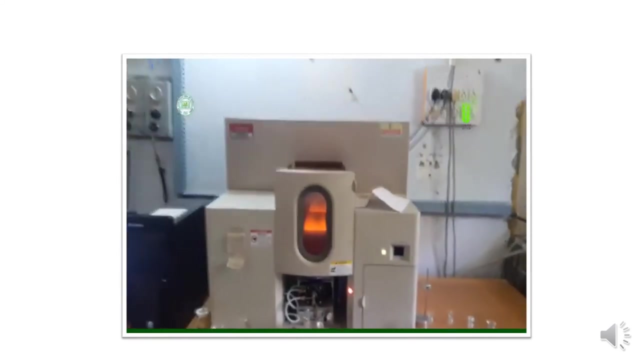 10 gram of soil into the manganese 125 ml allometric flask and add 10 ml extraction solution. dtp extraction solution we need to add. if we are using 5 gram soil, then we can add 10 ml extraction solution and if if we are using 10 gram soil, 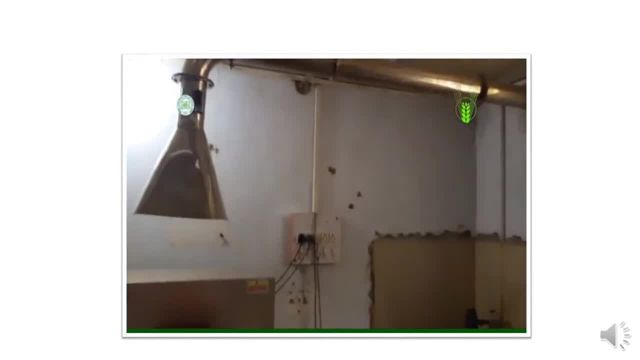 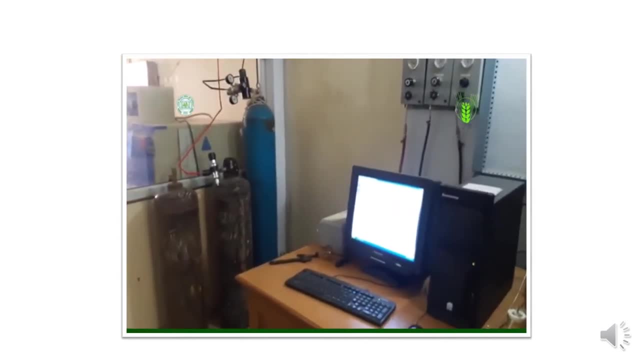 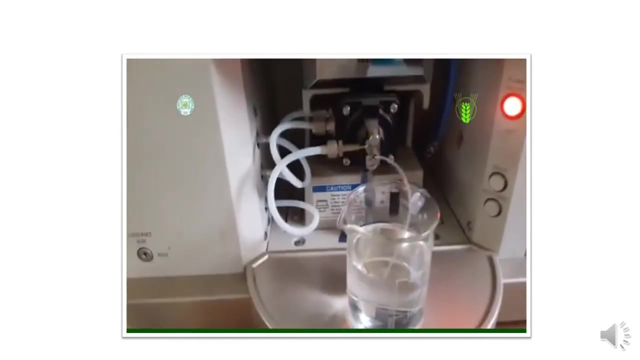 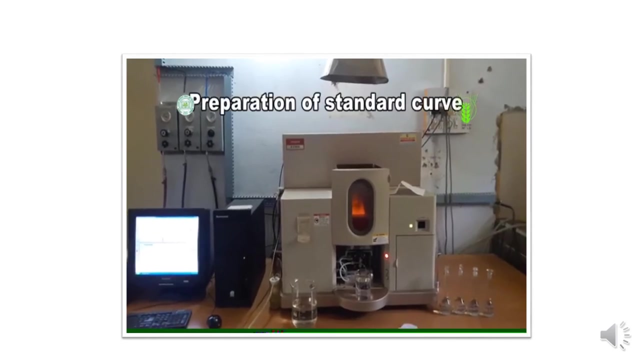 then we need to add 20 ml extraction solution. after adding the extraction solution, we need to shake it on the reciprocal shaker for 2 hours. After shaking, we need to filter the suspension through a filter paper. Now, after taking the filter, we need to analyze for the different 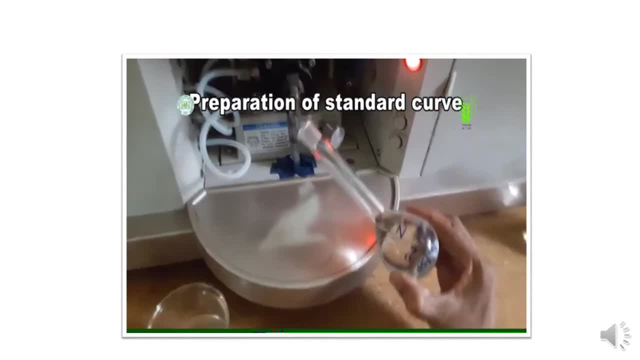 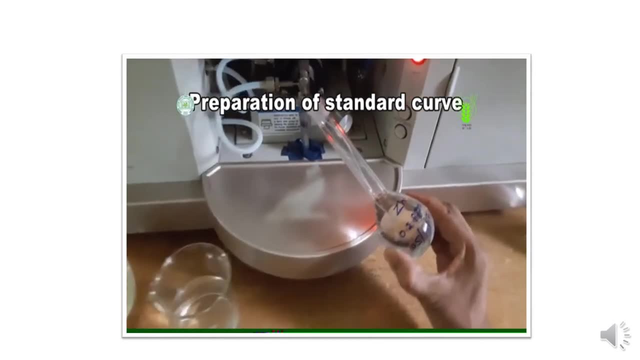 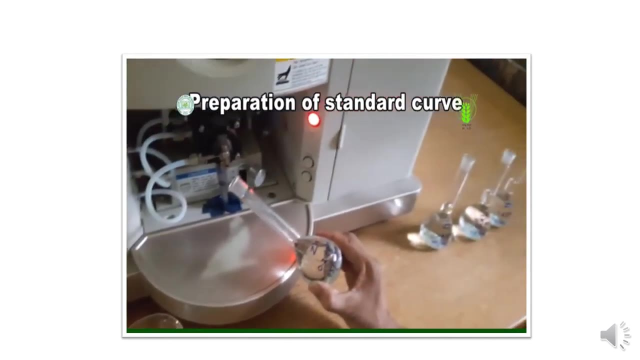 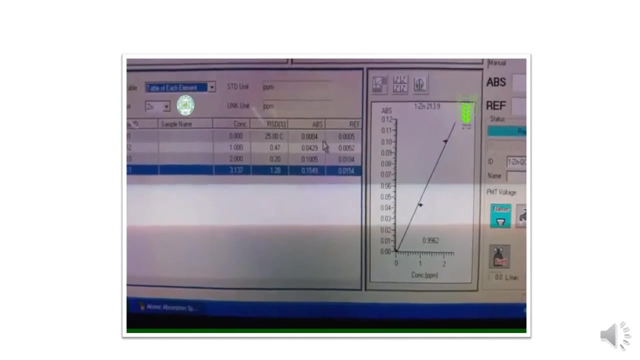 micronutrients. For the measurement of the zinc, copper, iron we need to operate atomic absorption spectrophotometer according to the instructions provided for the equipment. Here in the video you can see the atomic absorption. We will prepare the standard curve by using all 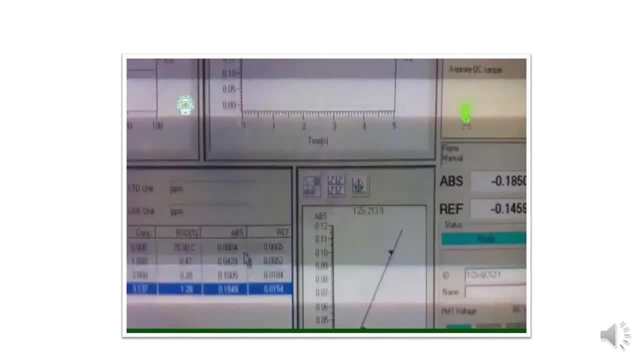 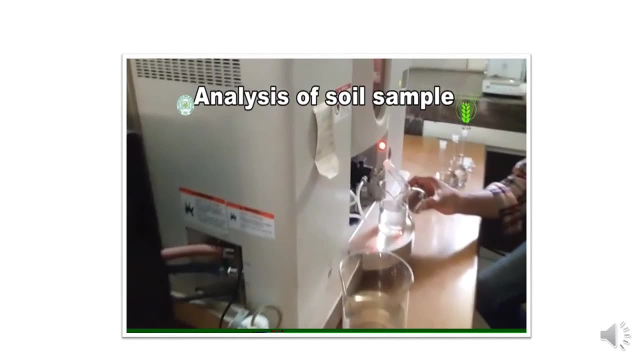 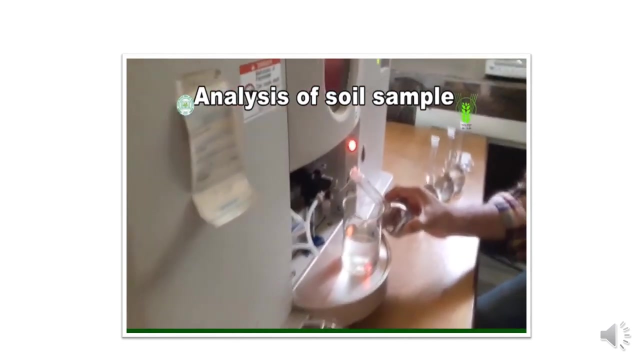 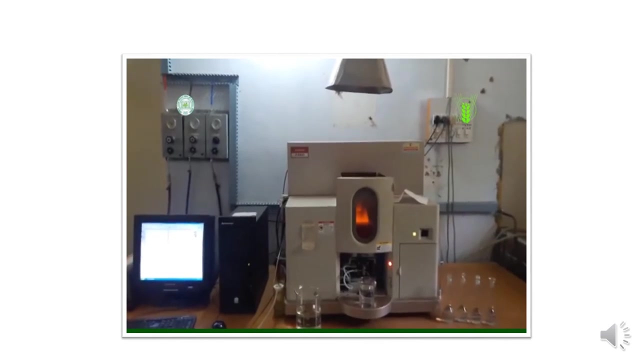 the series of the standard solution we prepared For each micronutrient. for zinc, we can see how we can measure the zinc. The atomic absorption will give the reading of absorption, because now we are running a series of standard solution And definitely we are going to draw a. 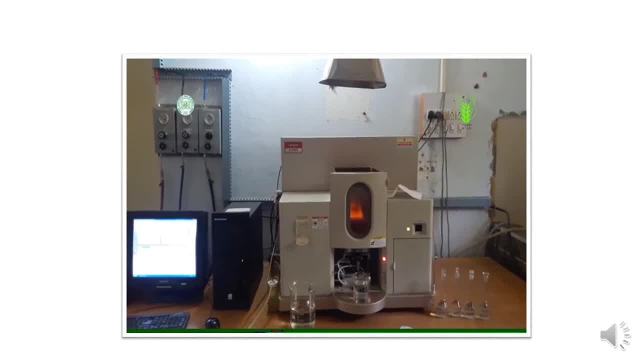 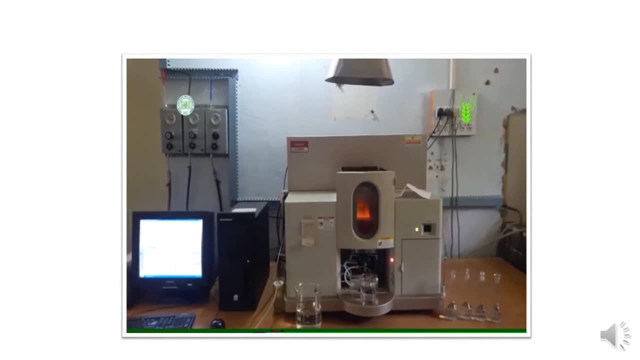 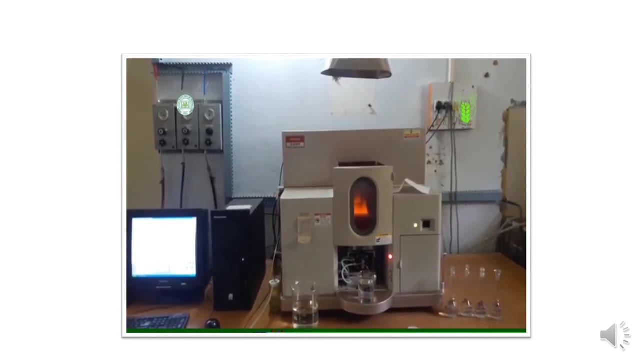 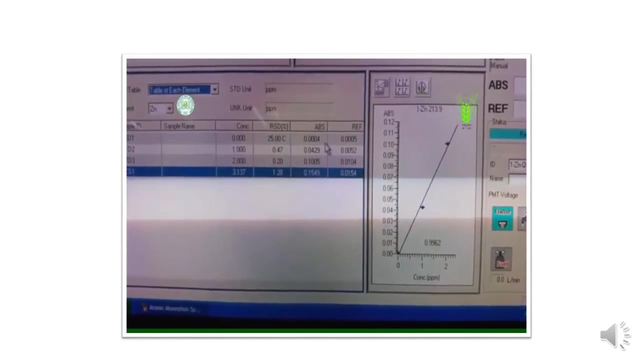 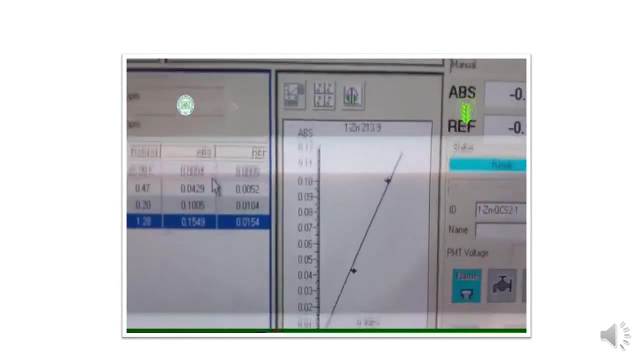 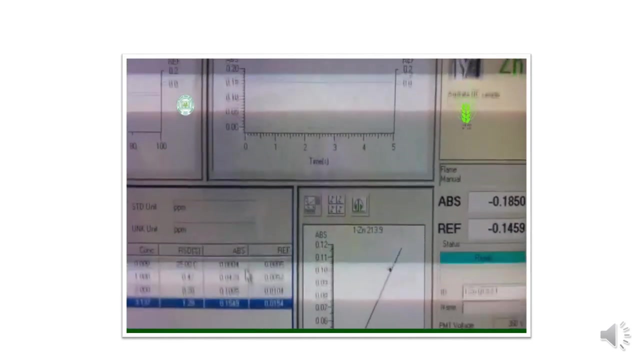 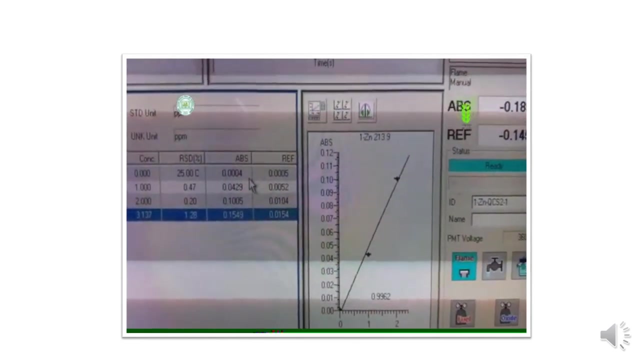 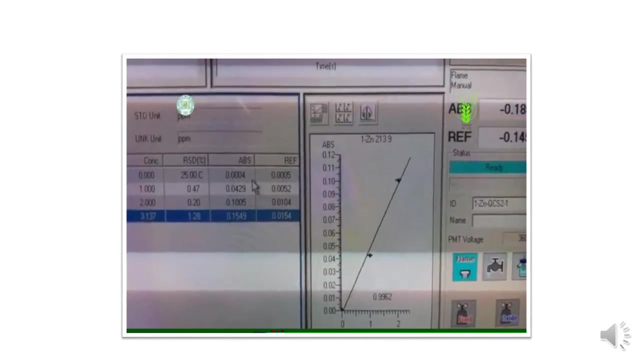 calibrated curve. Each standard solution for respective micronutrients will be run on the instrument. After drawing the standard curve, we will take the reading of the sample. After taking the reading of unknown sample or soil sample, its known concentration will be calculated from the standard curve. So the zinc concentration will be calculated. 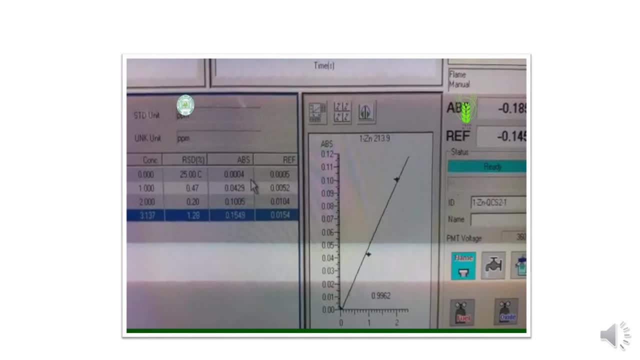 according to the calibration curve. Now let us have a look. I would like to mention that very important point here that, while atomic, for using the atomic absorption spectrophotometer, you must ensure that the particular lamp, a correct lamp for each element, because the specific element, the cathode lamp, is specific for each element. So you can see.